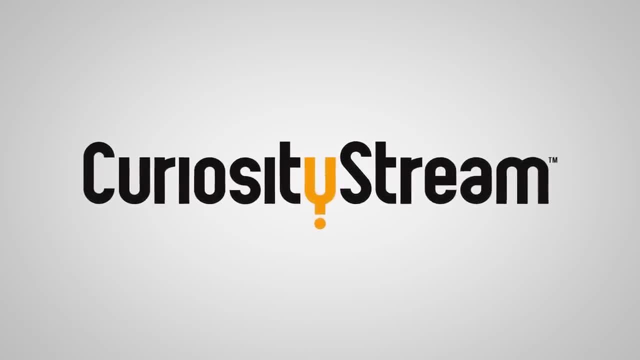 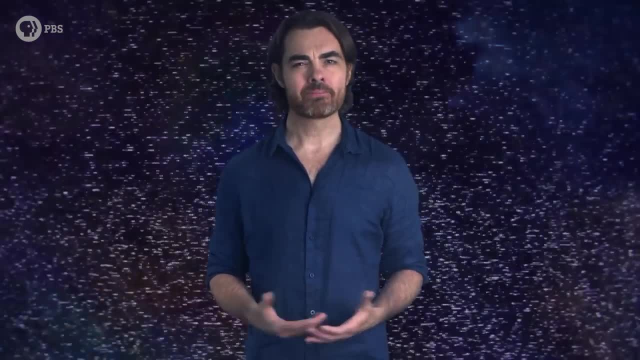 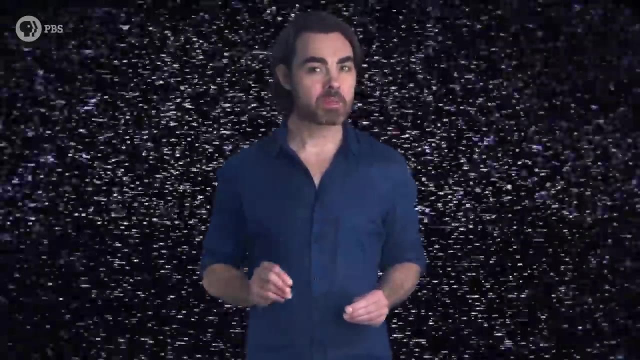 Thanks to CuriosityStream for supporting PBS Digital Studios. Hook up an old analog antenna to your TV and scan between the channels. That static buzz you hear is mostly due to the ambient radio produced by our noisy pre-galactic civilization. But around one percent of that buzz is something very different: It's the cosmic. 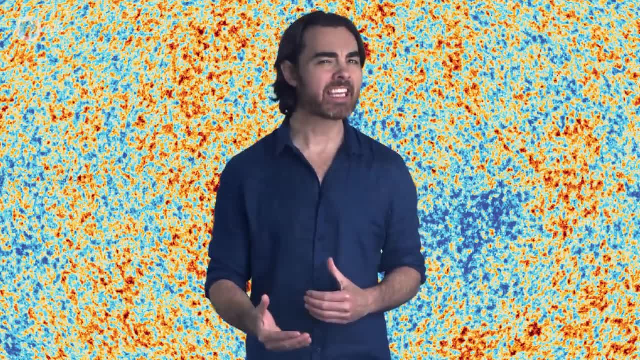 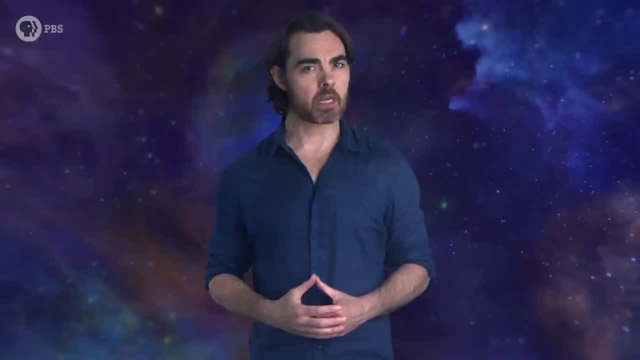 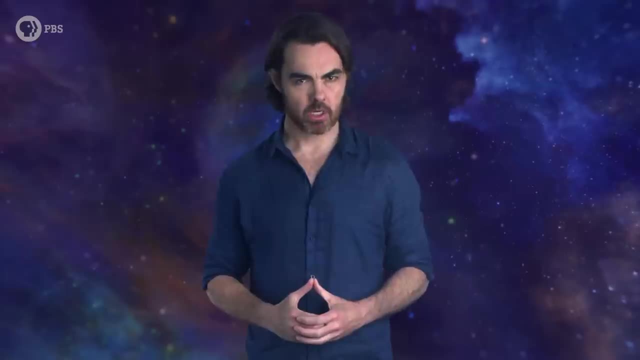 microwave background radiation, the remnants of the heat glow released when the hot, dense early universe became transparent for the first time. It sounds like random static, but that buzz contains an incredible wealth of hidden information. It holds the secrets to the composition of the universe and allows us to peer into its fiery beginning. 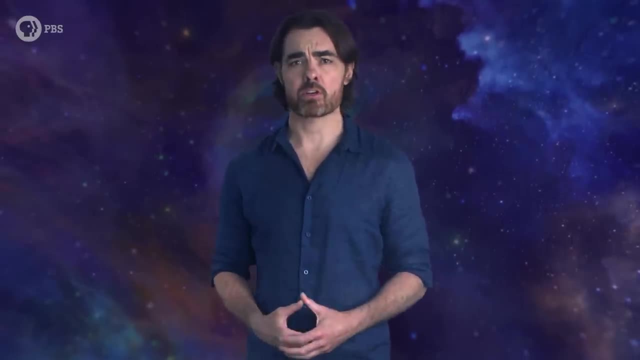 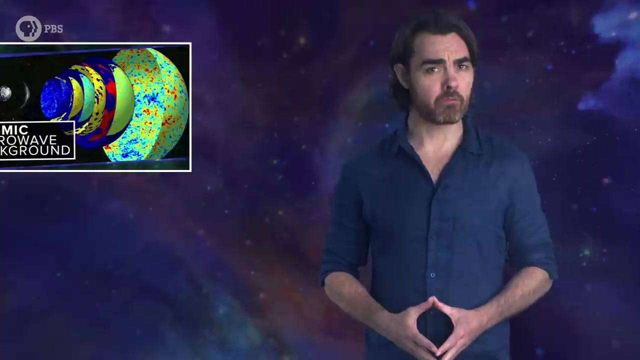 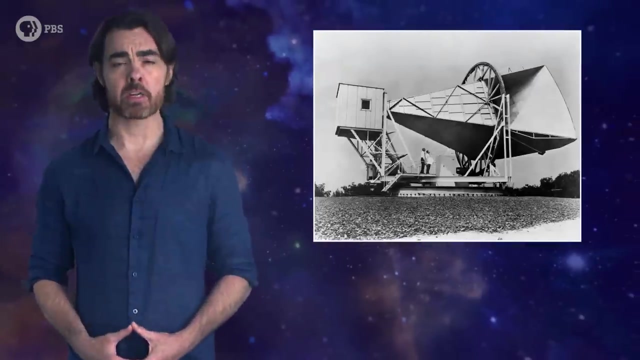 It's not surprising that scientists have spent half a century and built multiple satellites to unlock the mysteries of the cosmos, The cosmic microwave background. We've delved into its nature before, from its formation 380,000 years after the big bang to its 1964 discovery by Penzias and Wilson with the Holmdel horn antenna. 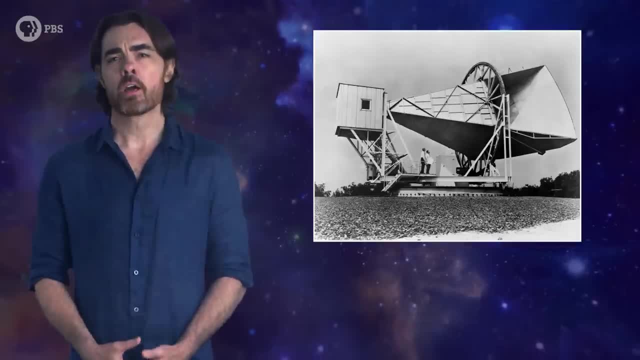 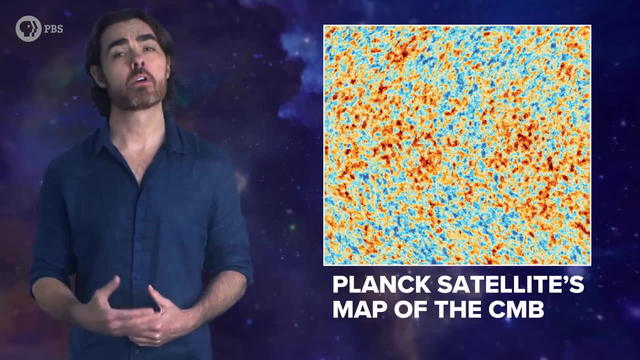 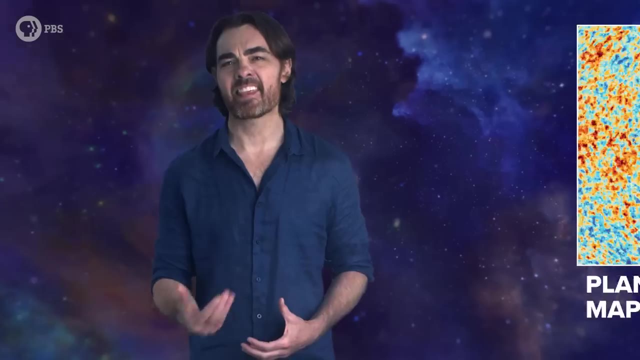 to its incredibly accurate mapping across the sky with ever better satellites. It all culminated in this: The Planck satellites map of the CMV. Those blotches are tiny differences in temperature Deviations of one part in 10,000 from the average temperature of only 2.7 kelvin. 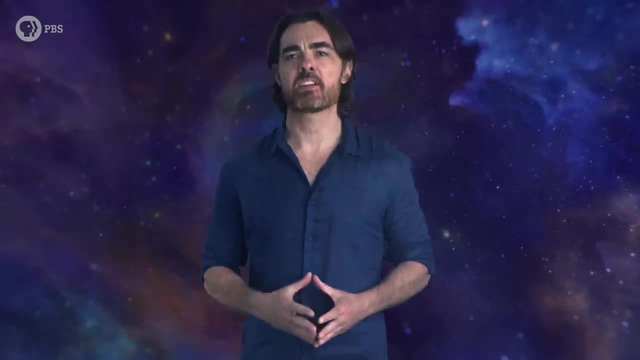 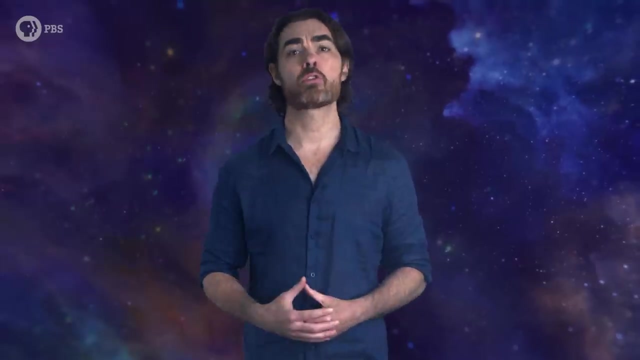 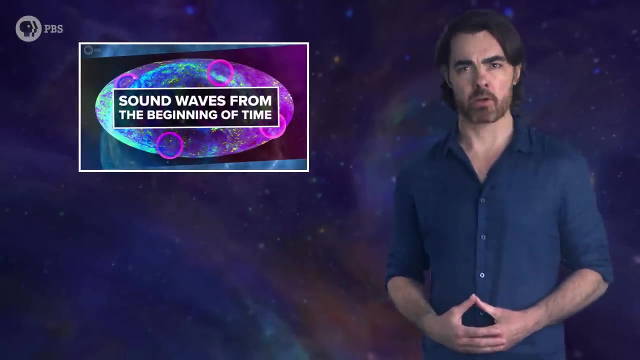 Those differences result from tiny variations in the density of matter right after the big bang, which evolved as colossal sound waves reverberated through the first few hundred thousand years of the universe's life. We explored these baryon acoustic oscillations in last week's episode, and that's really worth watching first if you haven't yet. 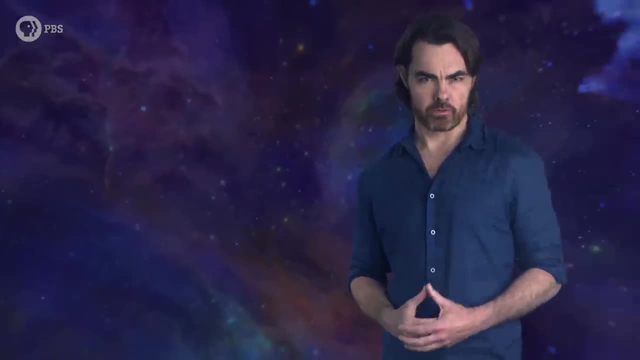 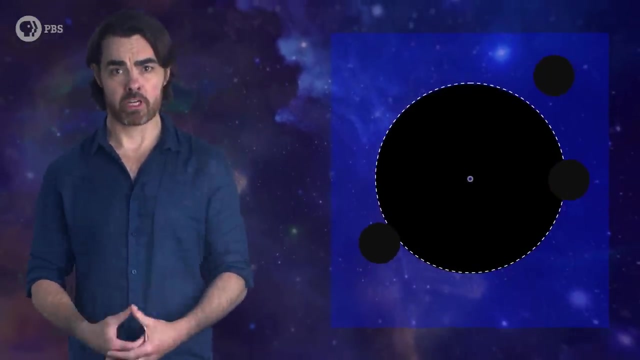 That episode painted a scene in the universe of the cosmic universe, but it's not the only one. A simplistic picture. A quick review. In the very beginning, dark matter flowed towards tiny regions of increased density drawn by gravity. Regular matter, what we call baryons, was in 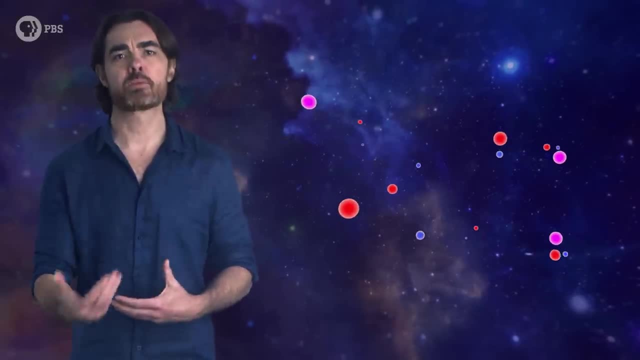 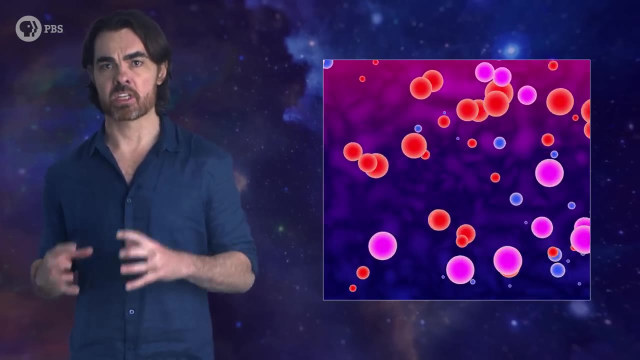 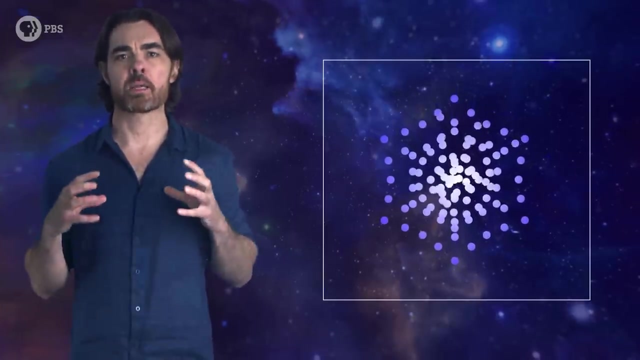 plasma form, with the simple atomic nuclei stripped of their electrons. in that extreme heat, In this plasma state, light and matter were locked together As the baryons compressed into over-dense regions. this led to a massive buildup of pressure. Collapsing baryons rebounded, producing an expanding sound wave, That expanding shell. 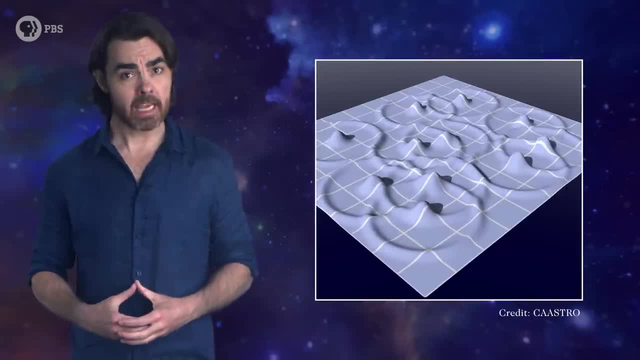 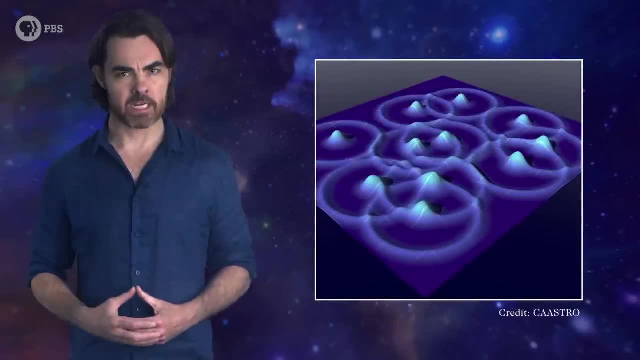 was eventually frozen in place. 380,000 years later, when light decoupled from matter at the formation of the first atoms, The moment of recombination. As the universe evolved, those frozen shells collapsed into galaxies. We still see them today. 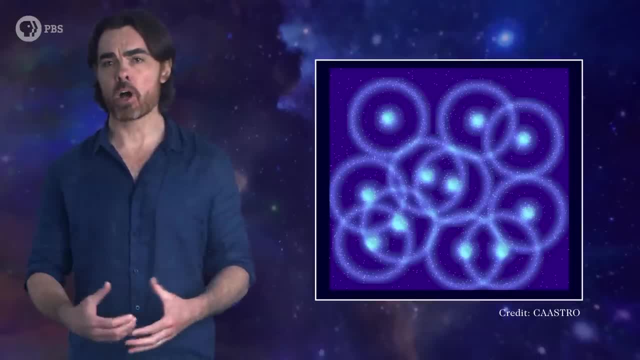 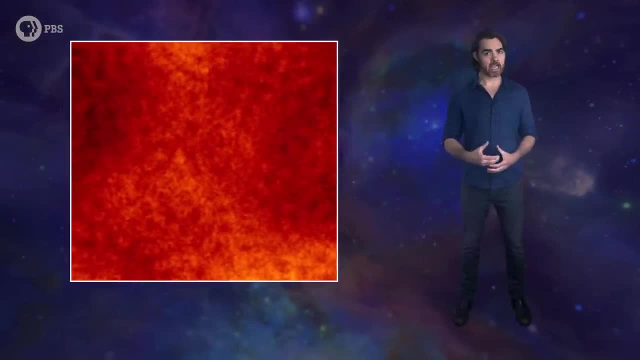 interwoven patterns of rings drawn in galaxies on the sky. But those rings are not the whole story. Today we're going to explore the intricate patterning not of the galaxies, but of the Cosmic Microwave Background Map, the image of the hot universe. 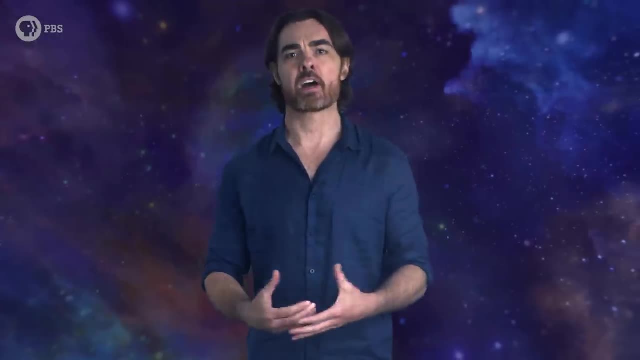 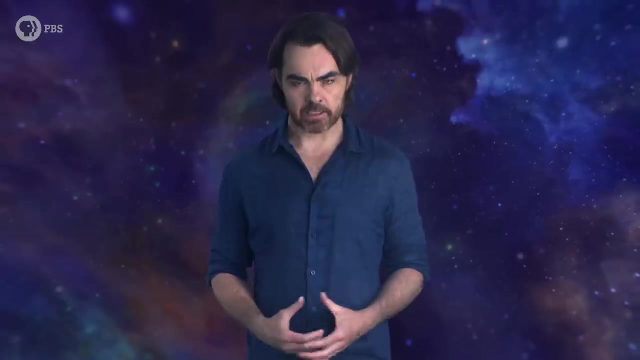 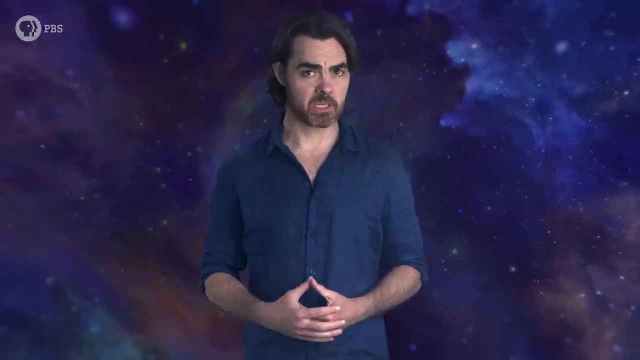 at the moment of recombination We'll see that the complex dynamics of the early universe are frozen into its spots. That patterning will tell us exactly what the universe is made of. As I said, this picture of a single expanding shell of plasma is simplistic In reality. 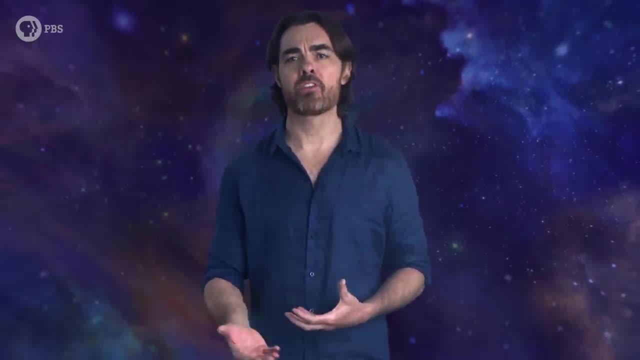 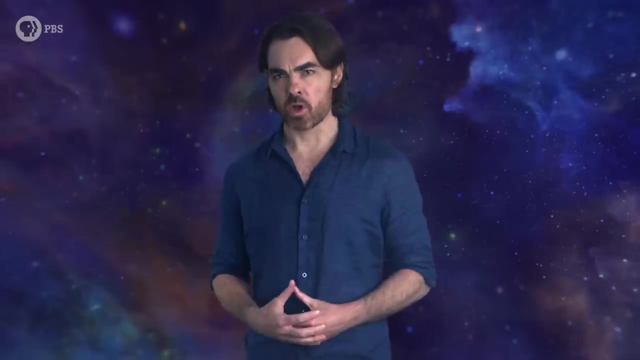 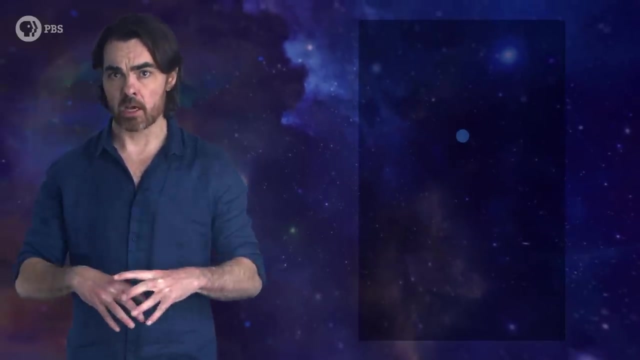 these acoustic waves pulsed in and out of their over-dense regions. They oscillated, and the number of oscillations depended on how large that over-density was. In some places, the over-densities were so large that matter only just had time to flow to the center. 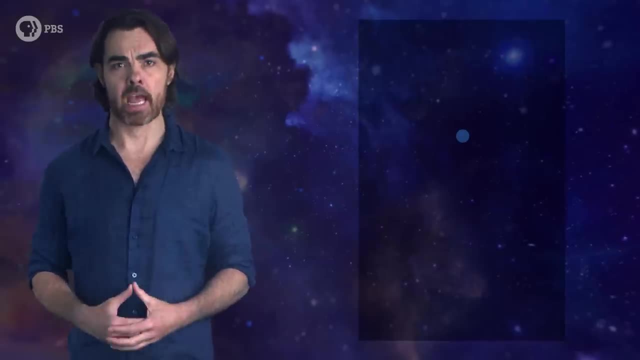 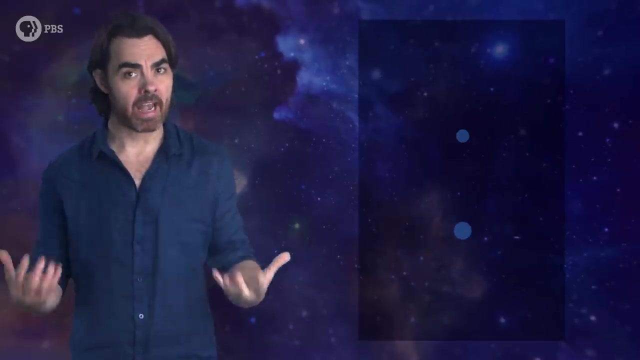 before being frozen in place by recombination. No rebounding happened And in other places the over-densities were smaller. The density wave had time to flow in, reverberate out and then get captured by the sun, The gravitational field once more falling back to the center. And that could happen. multiple times. Everywhere in the universe, the pull of gravity fought against the outward push of radiation pressure, causing density oscillations of all sizes. The state of those oscillations was then frozen at the moment of recombination. This messy, overlapping network of oscillations resulted in the spotty mess that is the map of the CMB. But crazily we can untangle. 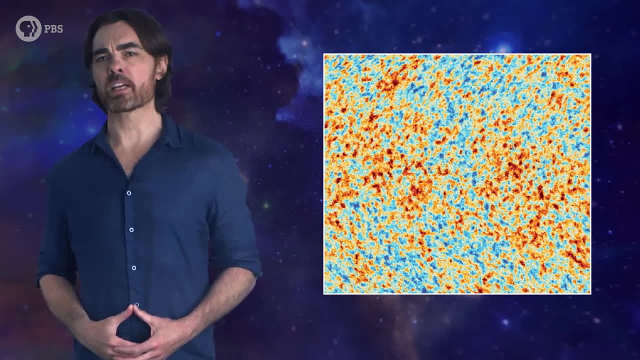 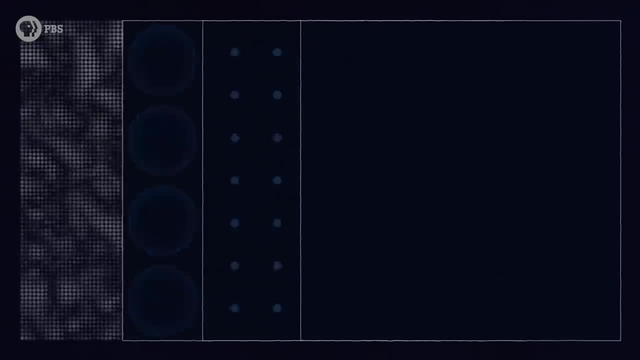 that mess. We can do that by thinking of these complex oscillations as just a bunch of very simple oscillations of all different sizes stacked on top of each other. This only works because the differences between the highest and lowest density regions are so small. So in our calculations we model the early universe as many overlapping layers. 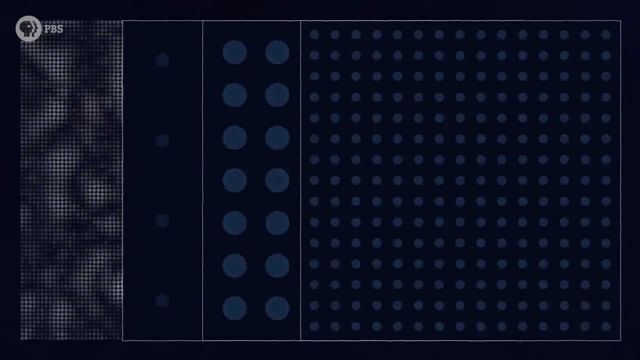 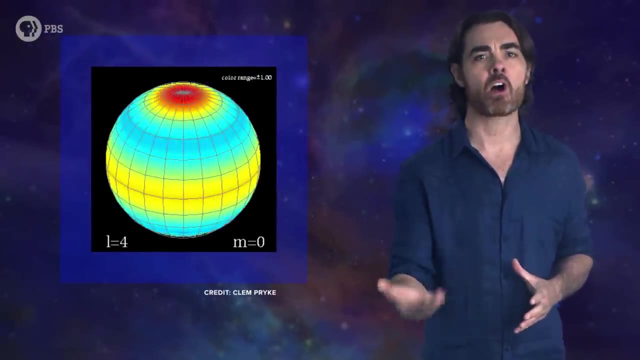 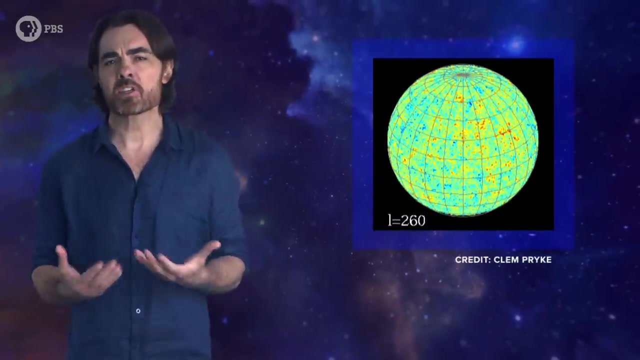 of simple density fluctuations. Each layer has fluctuations of a certain size, defined by the statics of spherical harmonics, Sort of like sine waves of different wavelengths, but on a 2D surface of a sphere, The fluctuations in each of these layers oscillates independently, But by 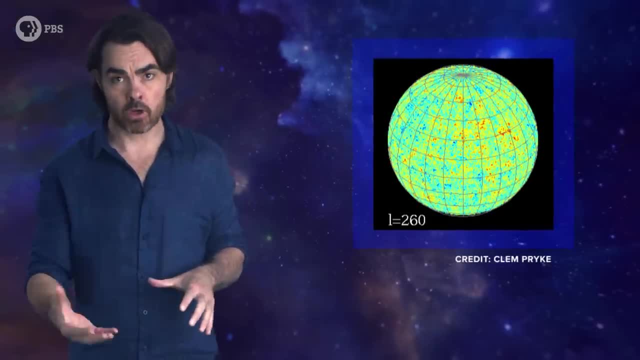 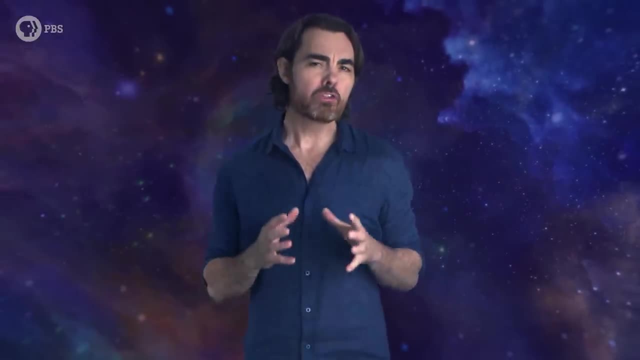 adding them together you can calculate the complex fluctuations of the early universe. Thinking about the oscillations this way leads to a really powerful prediction Over the 380,000 years between the Big Bang and recombination. each of our simple oscillations, basically. 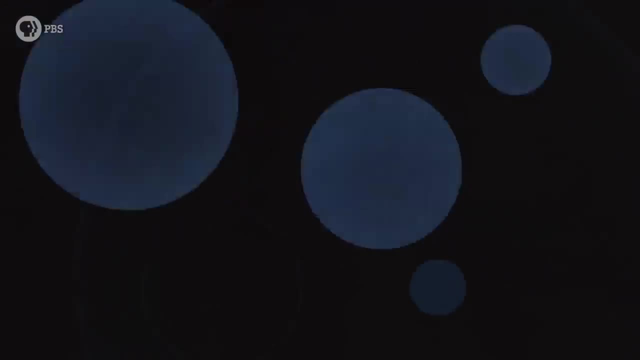 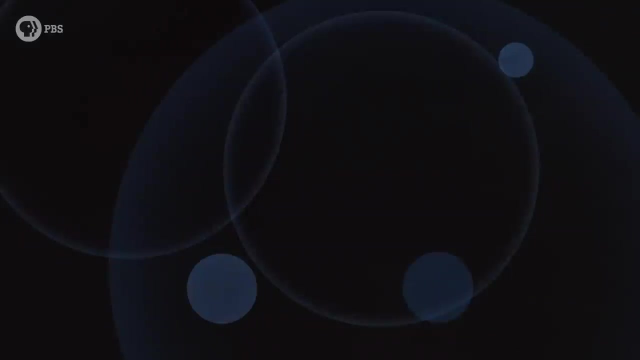 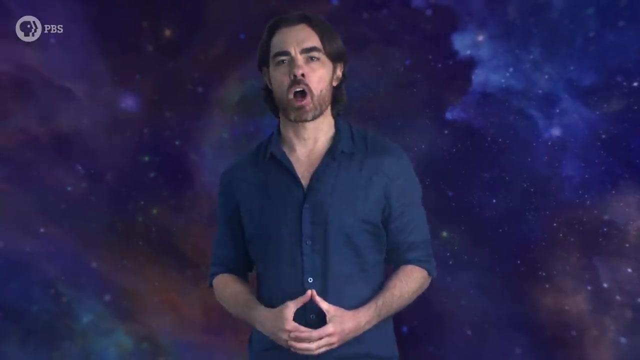 did its thing. Sound waves moved inwards, outwards, inwards, outwards. When recombination hit, most oscillators were caught in the middle of an in or an out flow. Those are not the interesting ones, But some oscillators- those with just the right size- were caught either at 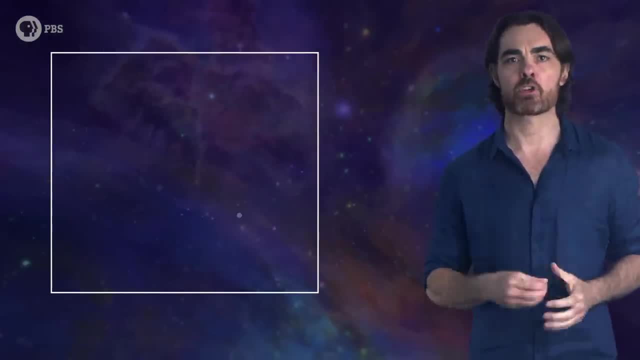 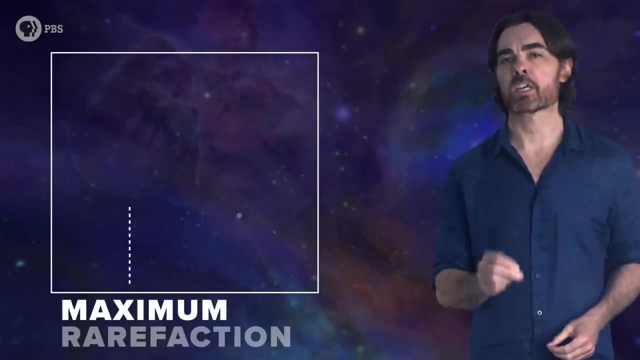 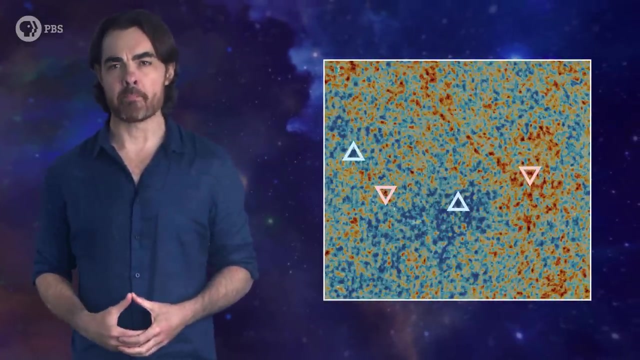 maximum density: matter concentrated in the middle of the fluctuation, or at minimum density with matter at its most spread out. We call that second one maximum rarefaction. These particular oscillations define the most obvious spots on the CMB map because they were frozen in their extreme states. So the most prominent spots on the CMB will have 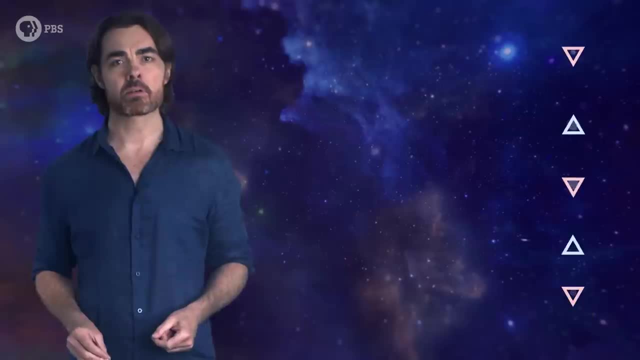 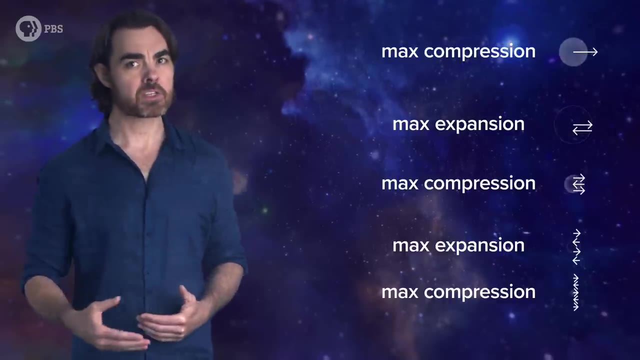 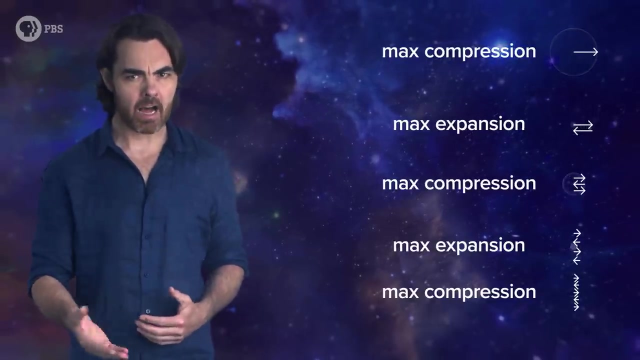 exactly the right size to get a single collapse, or one collapse, then an expansion, or two complete collapses, etc. The oscillations happened at the same speed- The speed of sound for our baryon photon, which was over half the speed of light. Okay, so we multiply the speed of sound. 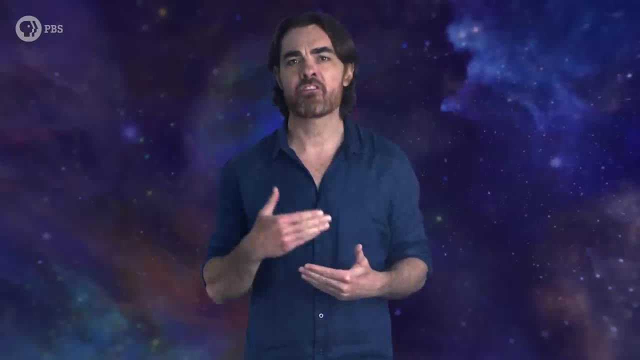 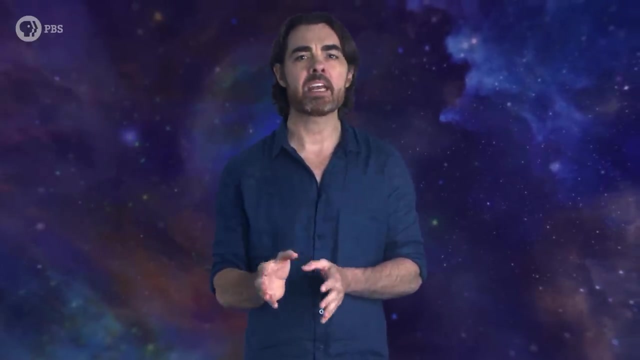 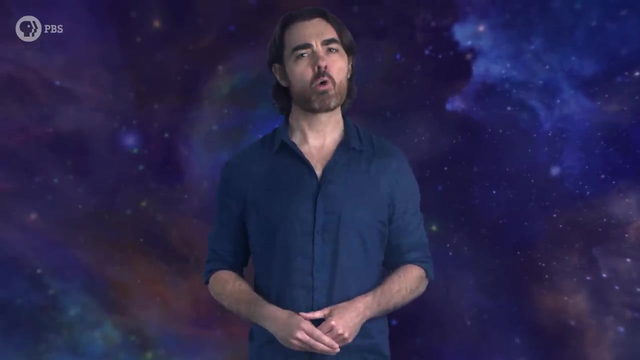 by the age of the universe at recombination. That's how far these density waves could travel. Divide that by the radius of a given density fluctuation and we get how many half oscillations it could execute. If the result is a whole number, then that fluctuation size will be at 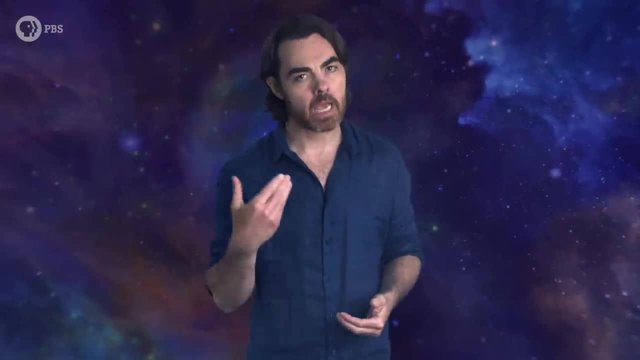 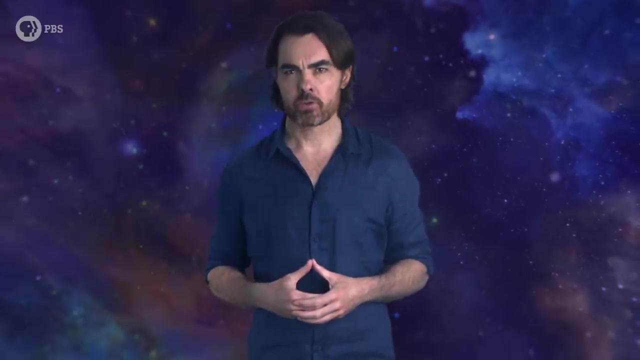 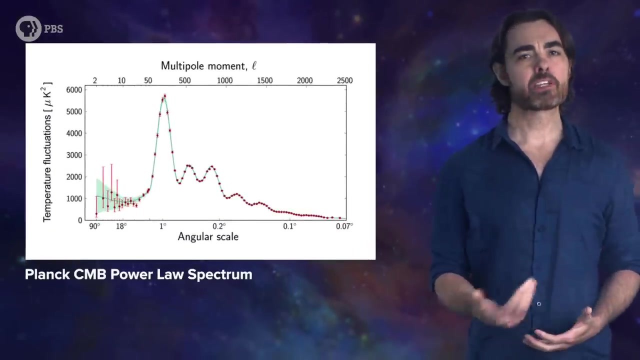 an extreme state- either all in or all out- at the moment of recombination. Now let's look at the first peak and we can see that the two largest sizes of these special spots should follow a harmonic series, And that's exactly what we see, The best way to show this. 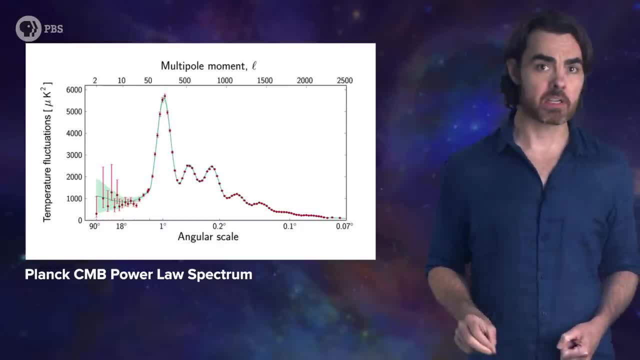 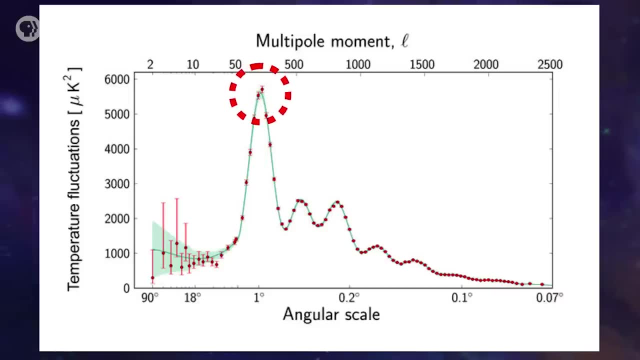 is with what we call a power spectrum. It's really just like a histogram that plots the number of spots of every possible size, And we definitely see that some sizes are more common than others. This peak here. those are spots in which the plasma only just had time to collapse. 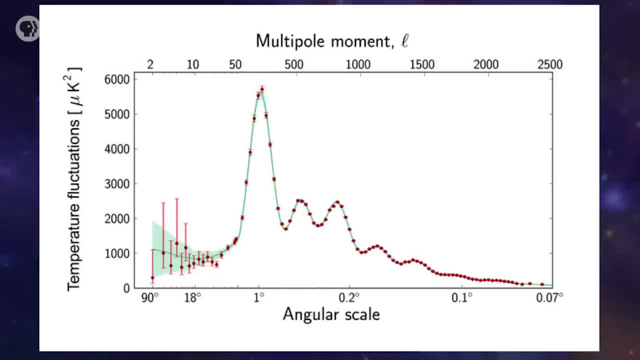 and we can see that the first peak corresponds to a full compression, then a full expansion. the third peak is for a compression, then expansion, then compression, and so on. Okay, nice, so we can explain the spot sizes, But what does this actually tell us about the universe? 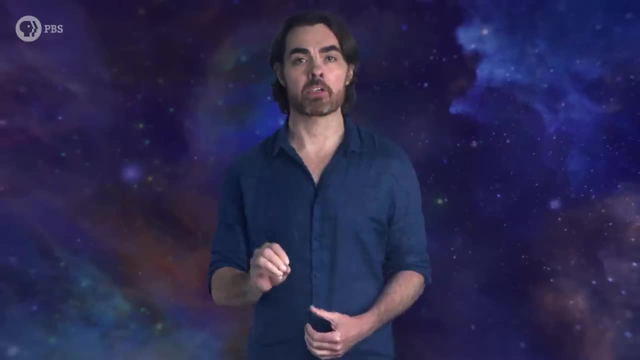 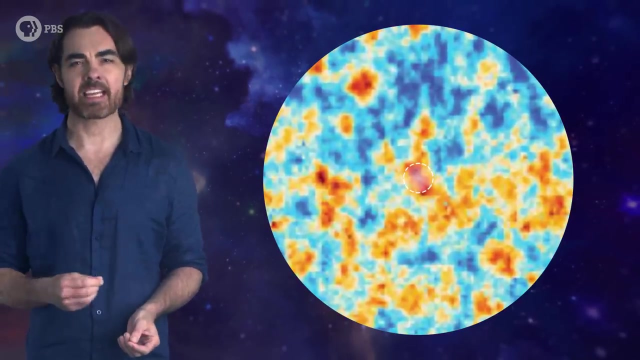 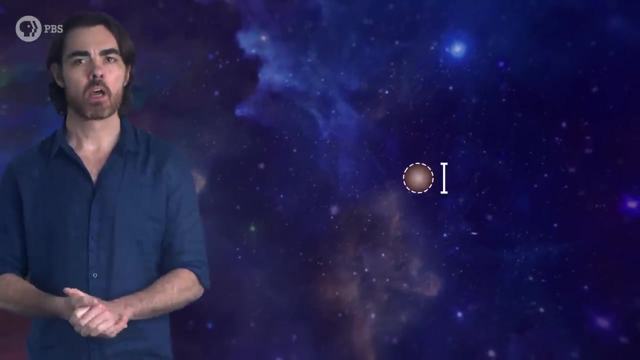 Well, kind of everything. In fact, each of these peaks tells us something unique. Let's go through them. The main value of that first peak is, as a measuring tape, Seriously, a standard ruler. This size represents fluctuations that had time to collapse exactly once, which means their size. 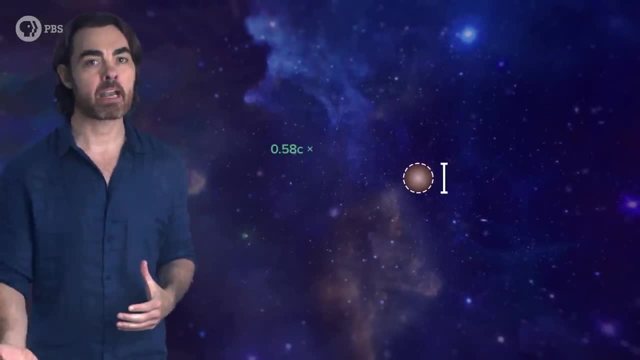 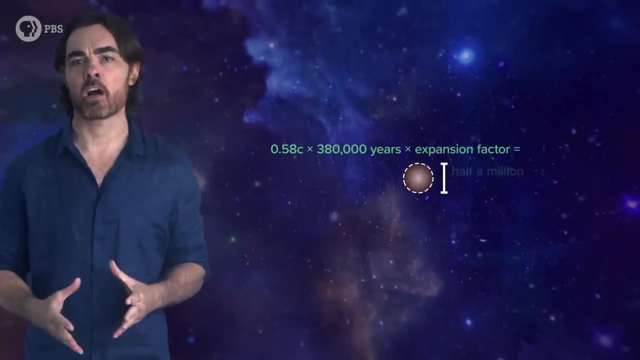 had to be equal to the speed of sound times, the amount of time that they had to collapse. Factoring in the expansion of the universe over that time, that size should be around half a million light years at recombination theoretically, And that gives us our ruler. 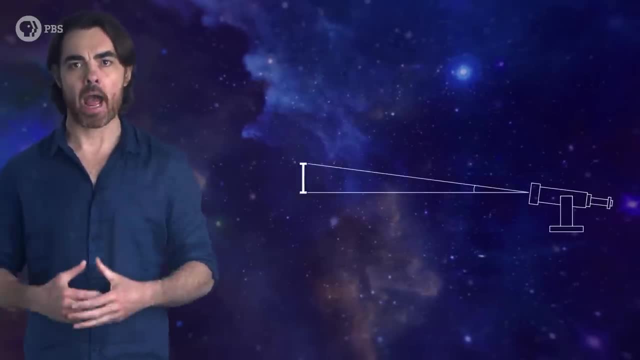 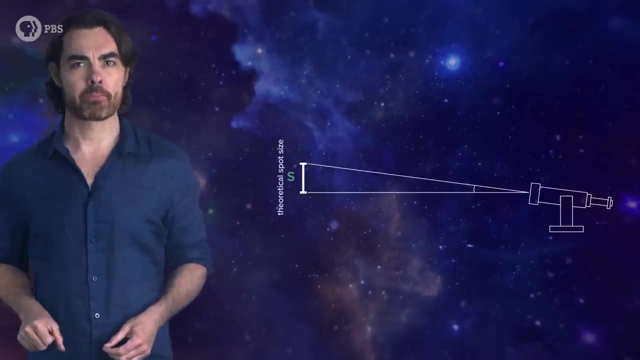 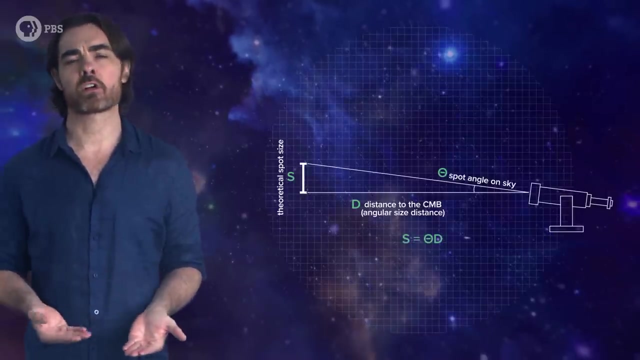 Now, when we try to measure the size of those spots on the sky, we actually measure an angle. We need to convert to a distance using trigonometry, And to do that we have to assume a flat universe. By flat I mean geometrically regular Parallel lines stay parallel and the angles of a triangle 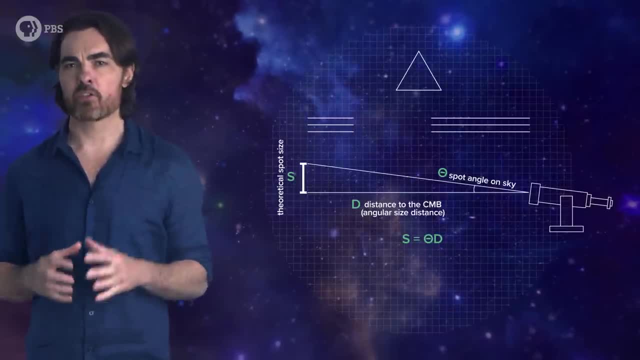 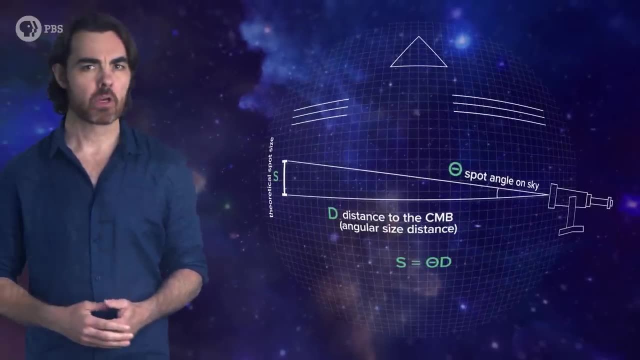 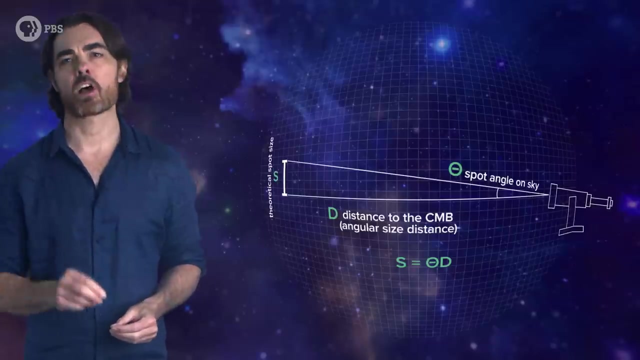 add up to 180 degrees. However, the presence of matter and energy, as well as cosmic expansion, cause geometry to be curved, which would mess up our basic trig. So here we have a test: If we measure the angular size of these spots and use simple geometry, 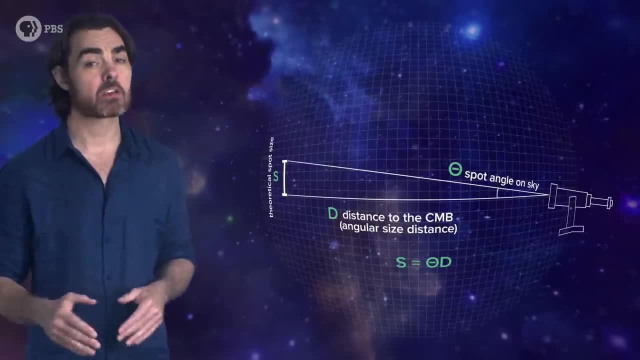 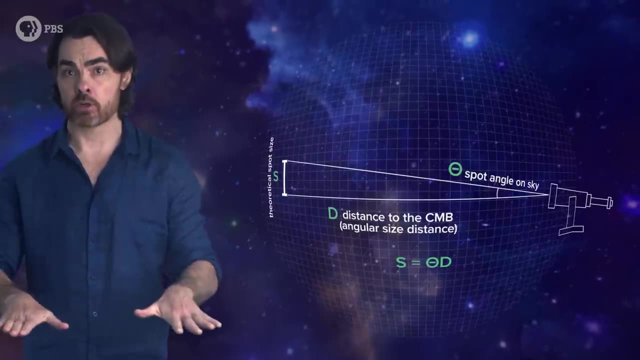 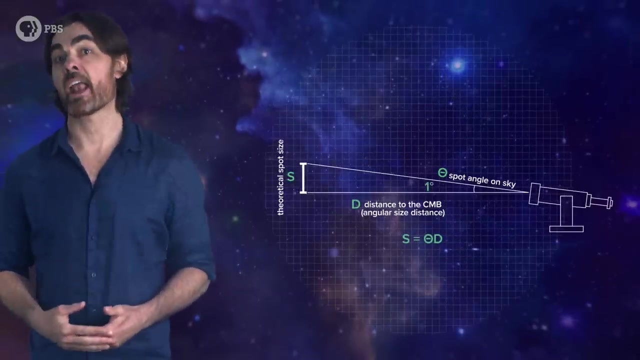 and that gives us the exact physical size that we expect from our theory, from our standard ruler, then that's a good indication that the universe is geometrically flat, And apparently it is. The spots are about one degree on the sky, which corresponds to that. 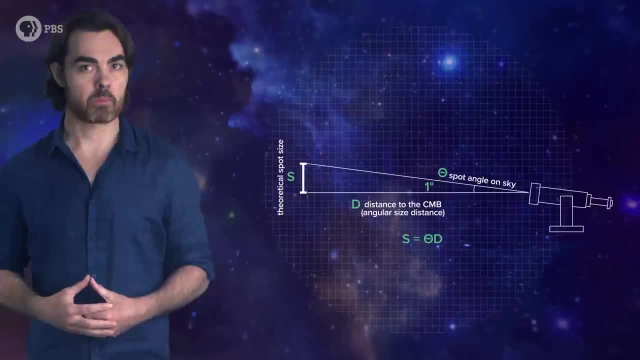 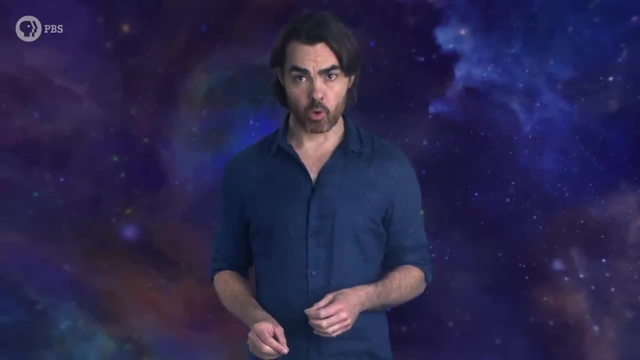 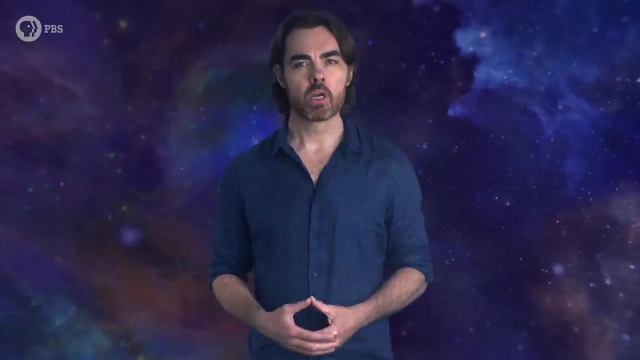 half a million light years that we got from the prediction To the limits of our ability to measure those sizes. the universe is flat. That tells us something very important. It tells us the total amount of energy in the universe. Energy results in positive curvature due to its positive 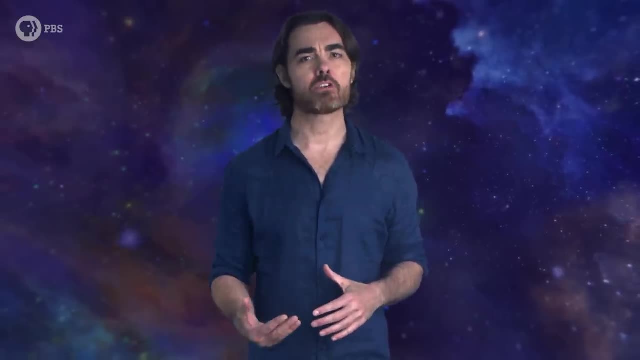 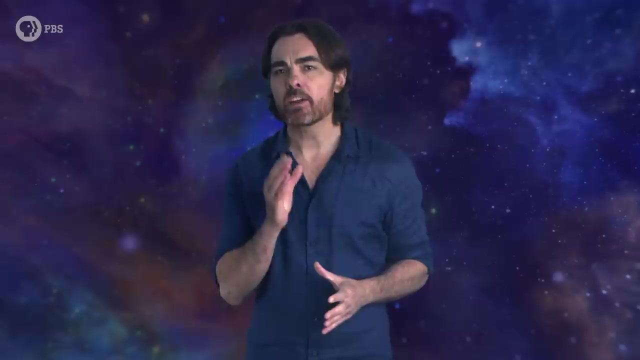 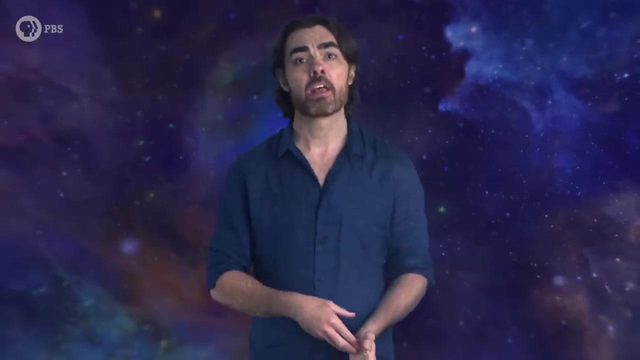 gravitational effect. On the other hand, an expanding universe with no energy would have negative curvature. So a flat universe must have exactly the right amount of energy to flatten the geometry of the universe. So that first, p tells us the universe is flat. therefore it tells us the total amount of energy, It tells us the sum total of baryons. 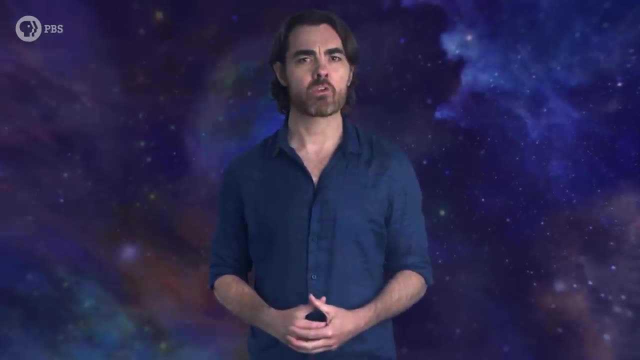 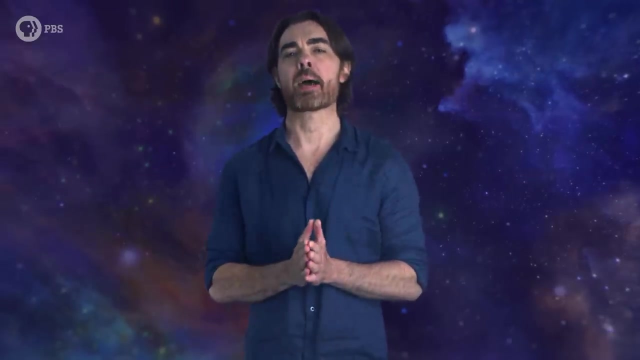 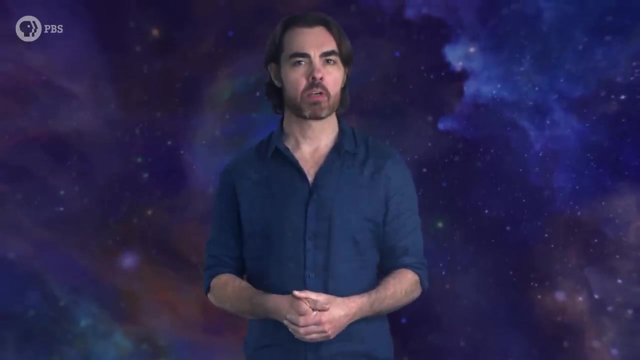 dark matter and dark energy. We'll see how useful that is when we look at the rest of the peaks. Okay, on to the second peak. That peak represents maximum rarefaction fluctuations where matter had fully bounced out once after its initial collapse. To understand the use of the second peak, 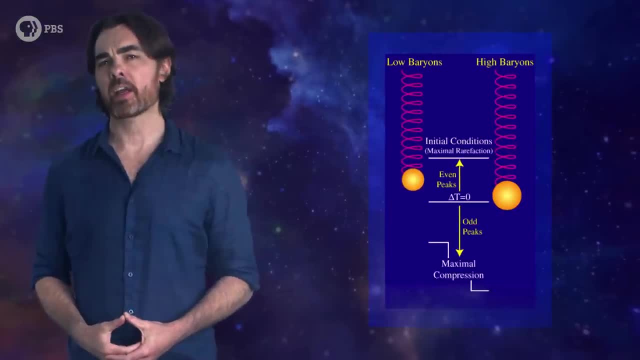 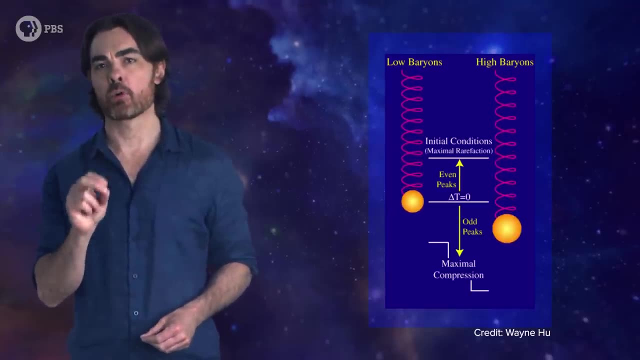 we need to use an analogy. We can think of these oscillations as being like a heavy mass attached to a spring. Release the mass and it falls and then bounces up again, always back to the original position, if it is a perfect spring. But the heavier the mass. 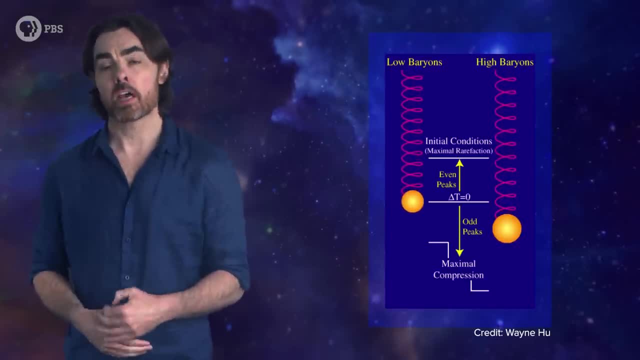 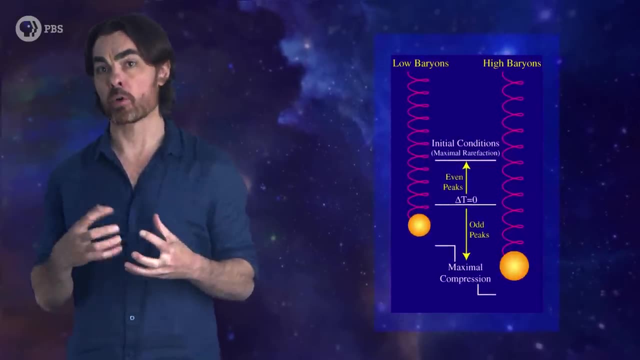 the further it'll fall before bouncing up. Maybe we had Seinfeld while racing around the moon, or maybe some sort of movie. Now think of the baryons as this mass. They're heavy and they want to fall towards our overdense spots, But the baryons are locked with light which act like our spring. 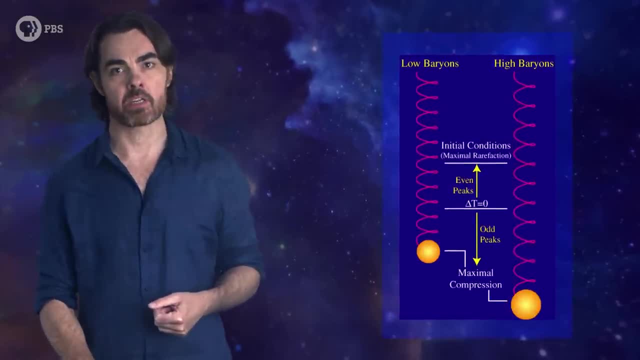 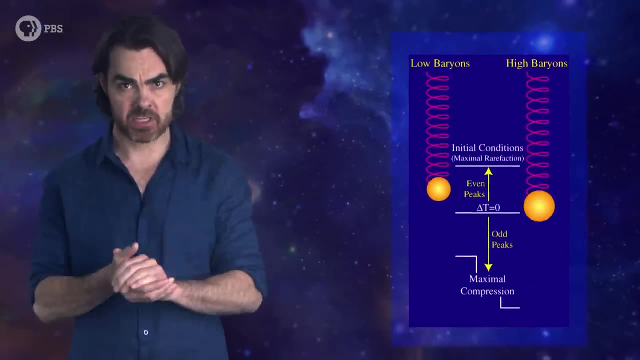 More baryons, deeper matter will fall into that overdensity. Having more baryons should the odd-numbered peaks, which represent the compressed state. On the other hand, the even-numbered peaks aren't directly affected by the baryons They represent. 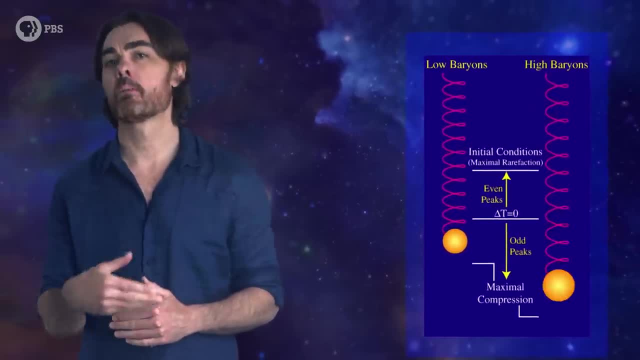 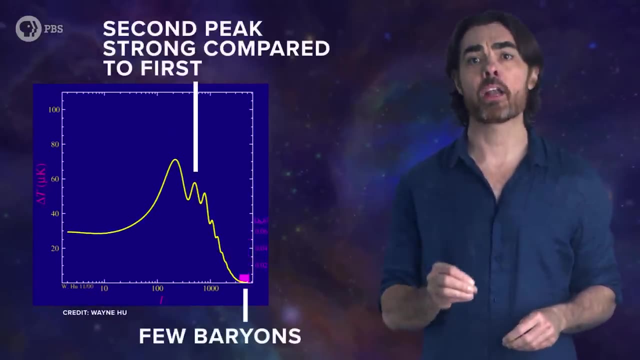 the top of the spring's rise, which is just determined by its starting position. What does this have to do with the second peak? Well, the more baryons, the higher the odd-numbered peaks are compared to the even-numbered peaks In. 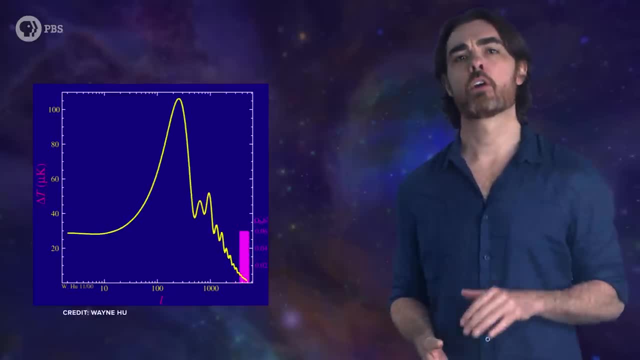 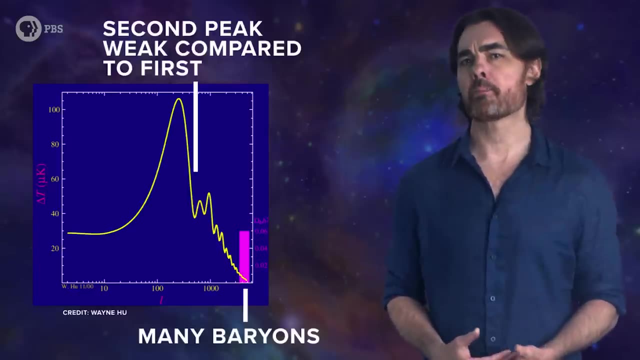 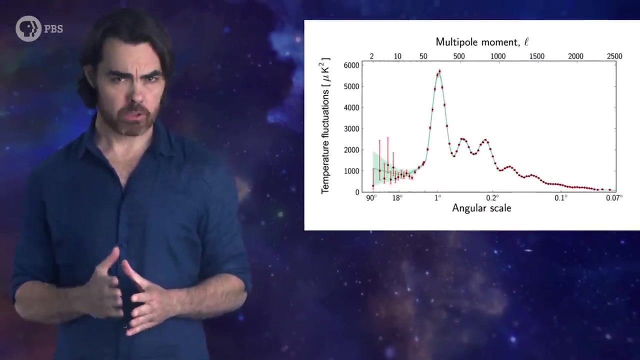 practice we can just use the height of the second peak relative to the first peak to measure the baryon content of the universe, And those measurements tell us that the baryons constitute only about 5% of the total energy of the universe. And finally we get to the other peaks, which represent the smallest. 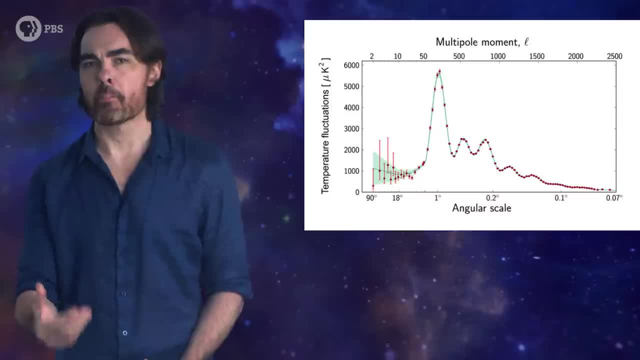 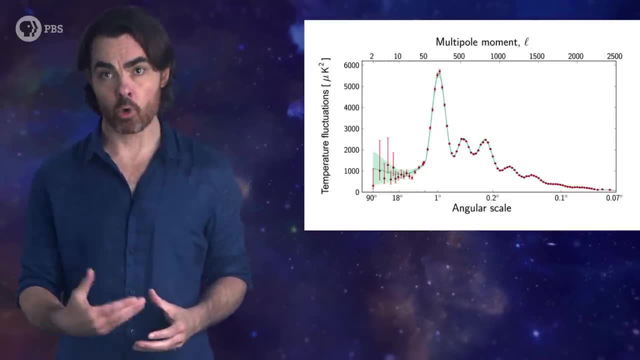 fluctuations. These tell us about the dark matter. Well, more accurately, they tell us about the relative amount of dark matter compared to radiation or light. Now, this is a bit too much of a rabbit hole for right now, but, in short, in the 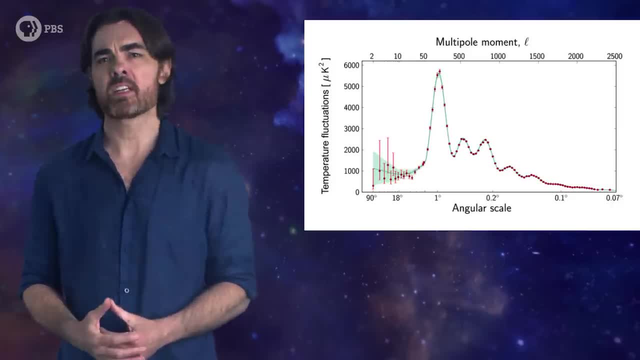 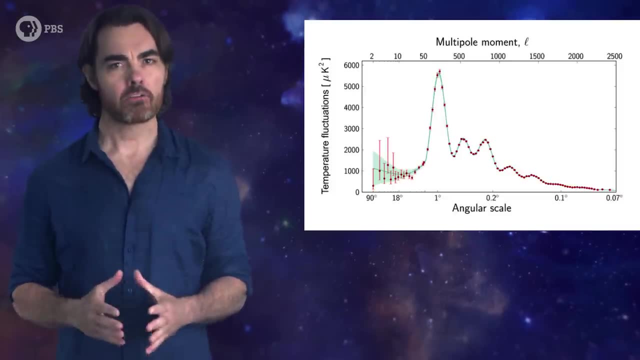 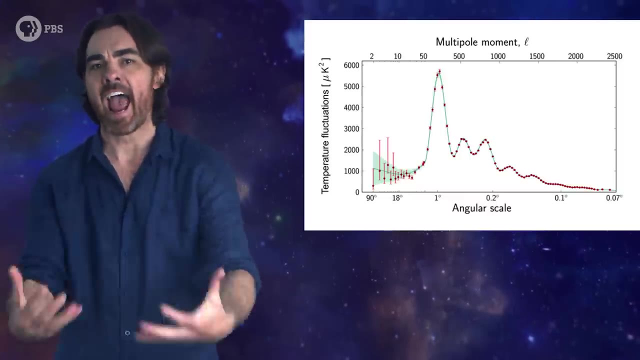 first few tens of thousands of years, the universe was in the radiation-dominated epoch. Basically, photons produce more gravity than matter. Fluctuations that were small enough to oscillate at least once during this brief time should be enhanced. Their peaks on the power spectrum should be raised compared to 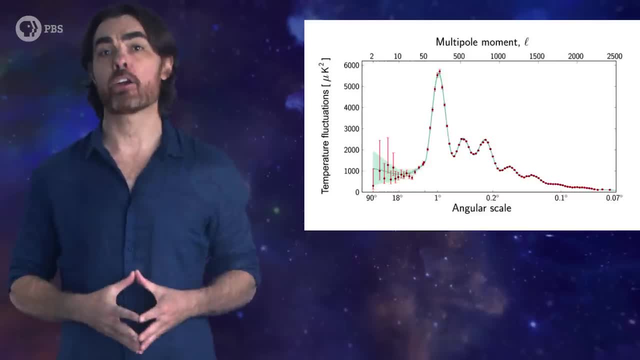 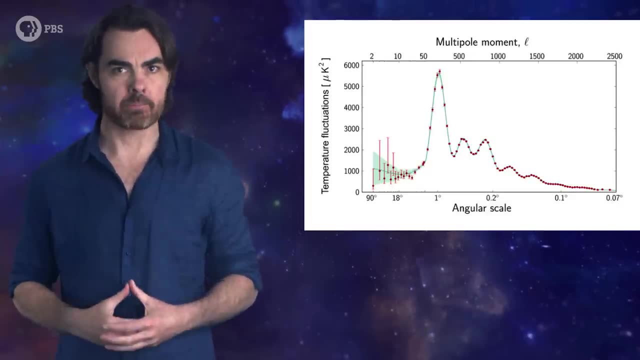 the larger fluctuations. So by looking at the height of those smaller peaks you can actually figure out when the radiation epoch gave way to the dark matter-dominated epoch. That in turn tells you how much dark matter there is. there's a lot. 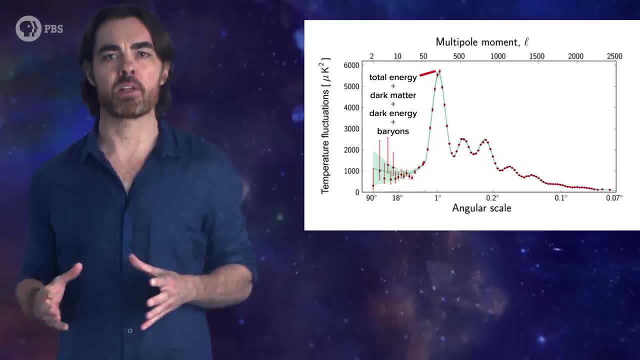 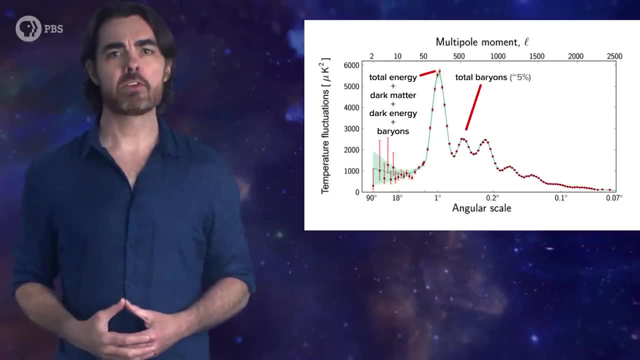 OK, let's bring all this together. The size of the spots in the first peak tells you the total amount of dark energy, dark matter and baryons. The second peak gives you just the amount of baryons, And the higher peaks give you the amount of dark. 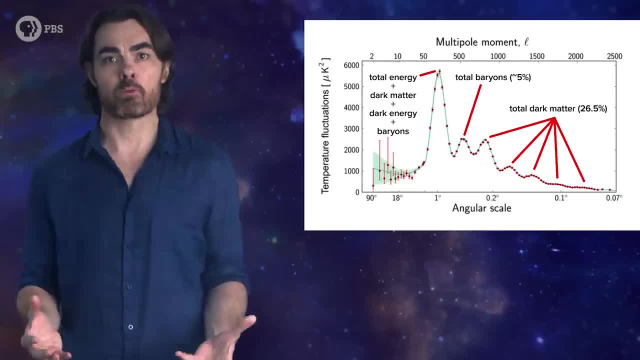 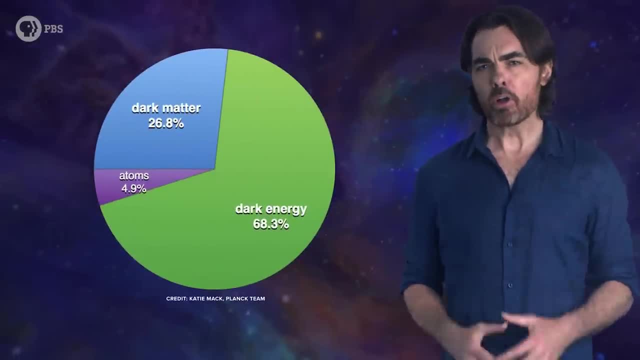 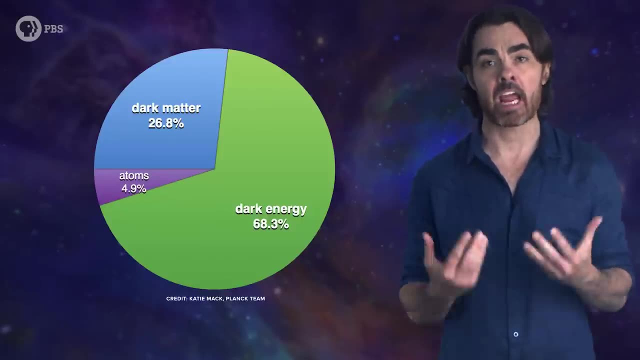 matter. Combining this, we can separate the relative contents of all three components. extrapolate that to the modern universe and we get that baryons constitute only 5% of the mass and energy. That's all of the atoms in all of the stars, in all of the galaxies, basically everything. 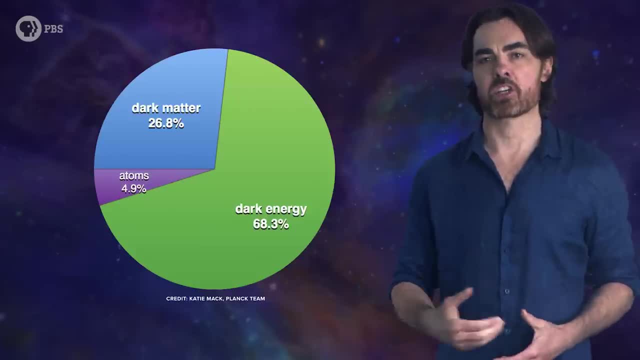 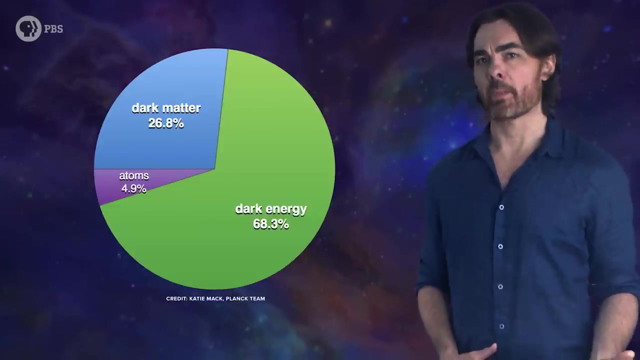 you can see. The remaining 95% is the so-called dark sector. Dark matter is 26.5% and dark energy is a whopping 68.5%. This is a super important verification because we get approximately the same numbers when we look at the dark matter content in modern galaxies and clusters. 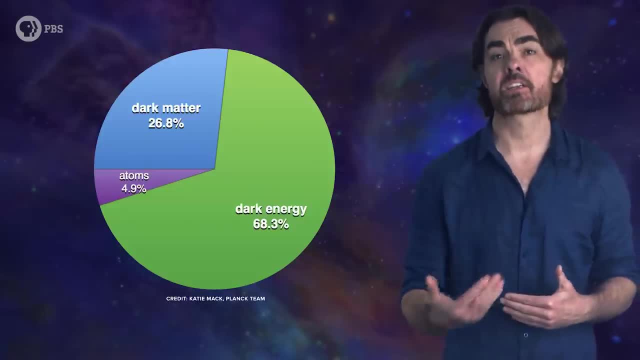 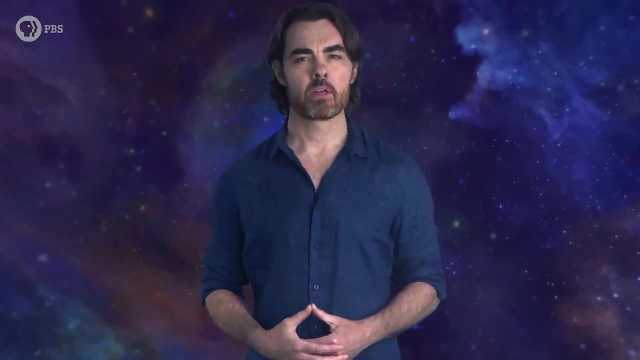 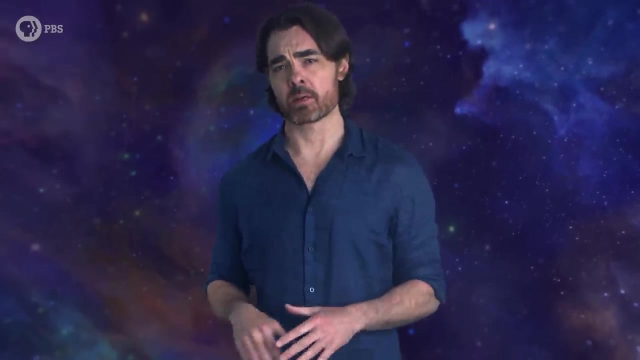 and the dark energy, based on measuring the accelerating expansion rate of the universe. So that's how you lay bare the secrets of the cosmic microwave background. It's an insane wealth of information from what looks like random, minuscule fluctuations in this faint, noisy bubble. 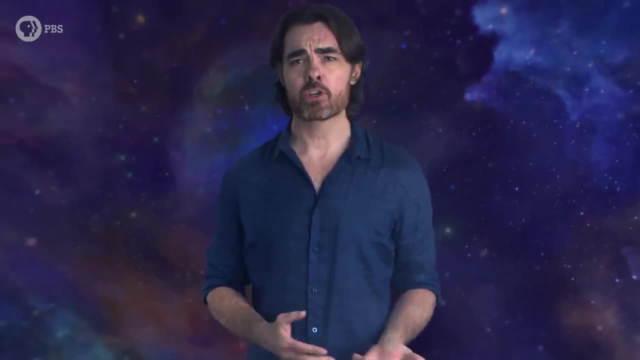 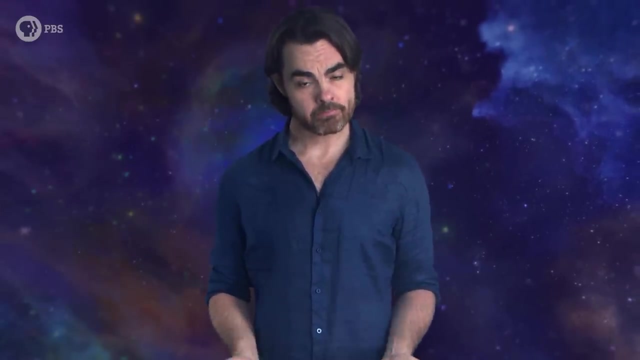 So next time you hear the static whisper of an untuned TV or radio, remember that in that noise can be found the secrets of the earliest epochs of space-time. Thank you to CuriosityStream for supporting PBS Digital Studios. CuriosityStream is a subscription. 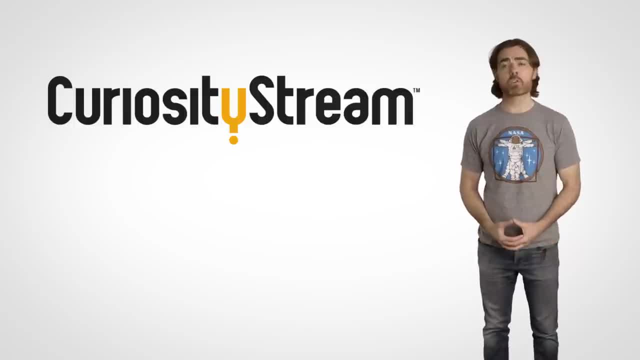 streaming service that offers documentaries and non-fiction titles from a variety of filmmakers, including CuriosityStream originals. For example, you can check out The Joy of Chance, which explores whether chance is a fundamental part of the universe, And it probes whether chance has rules You can learn. 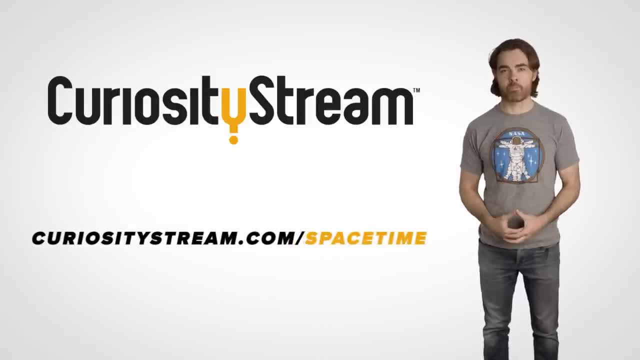 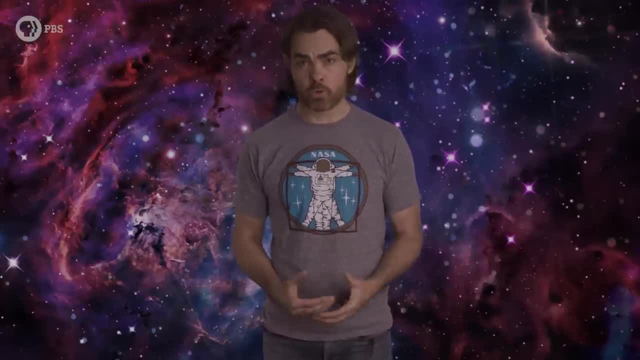 more at curiositystreamcom slash spacetime. In our previous episode we started our discussion of the baryon acoustic oscillations, the actual source of the CMB power spectrum. Let's see what you guys had to say: Flux, Capacitor and Marcus. 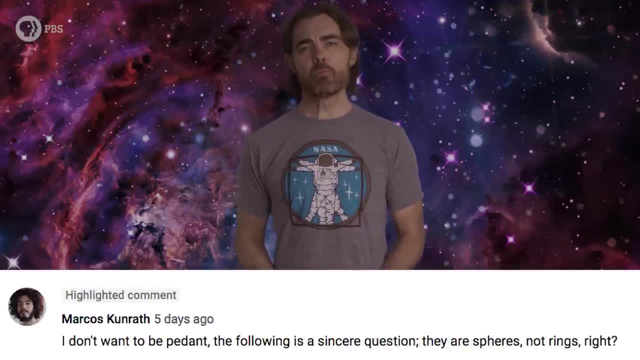 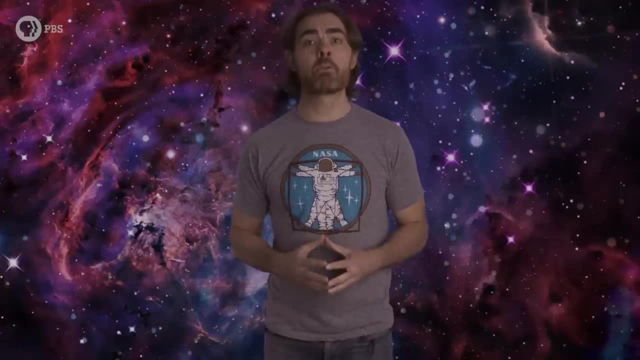 Kunrath point out that the baryon acoustic oscillations should have produced bubbles, spheres, rather than rings on the sky. That's right. They definitely would have produced 3D spherical shells, not rings. Sorry if I wasn't clear about that, So you should actually have overlapping. 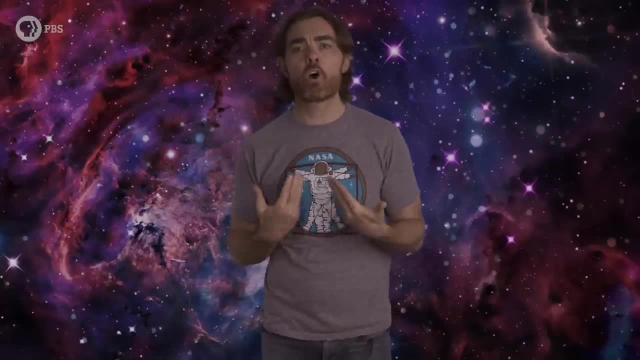 bubbles of galaxies throughout the universe, But we only see a 2D projection of that universe. When we look through the edges of those bubbles, we see many more galaxies compared to when we look through the thin layer at the middle of the bubble. 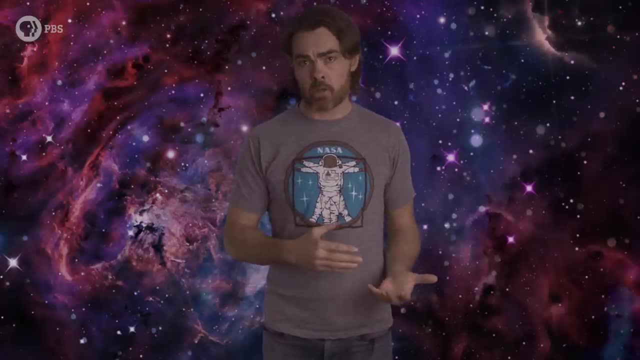 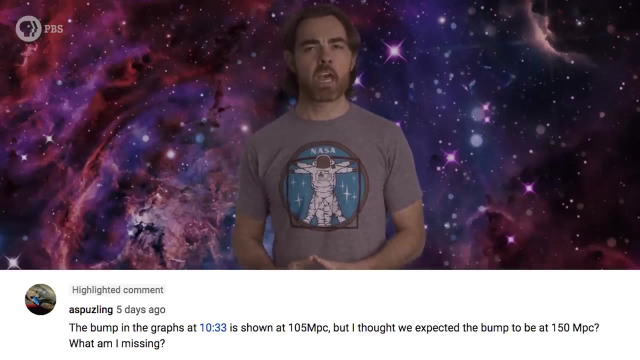 It's just like when you look at soap bubbles: The edge is darker than the center. As puzzling, notice that the graph of the CMB power spectrum has a first peak at 105 megaparsecs rather than 150 megaparsecs, which is the size I actually stated The reason. 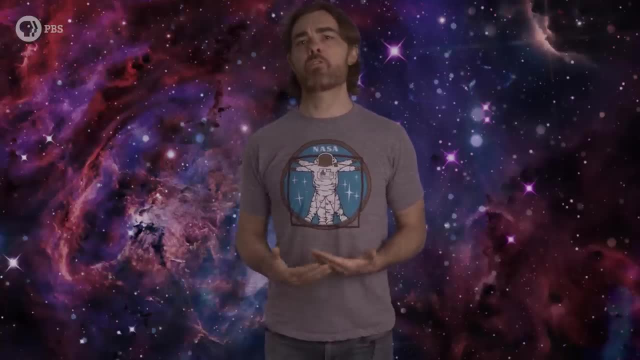 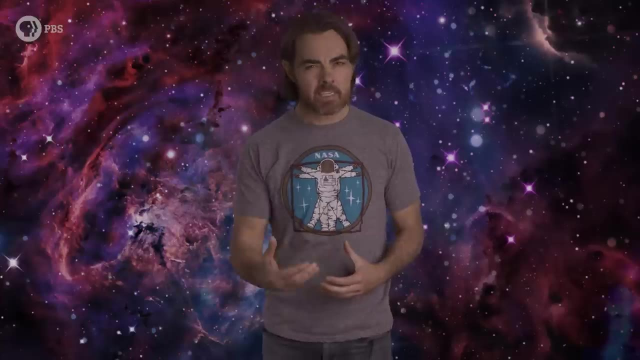 for this is that the authors of that paper use a different value for the Hubble constant. See the quoted distance is the co-moving distance. It's the size of the distance, thePHEV I'd size the ring would have if it existed in the modern universe, given the rate of expansion. 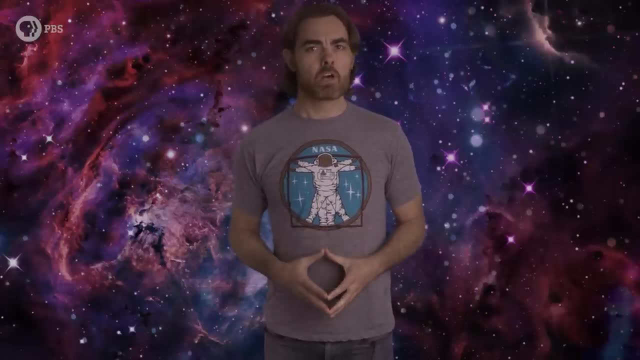 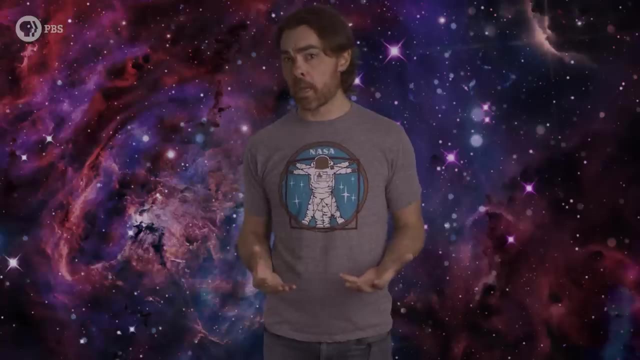 of the universe. The surveys that measure these rings look so far in distance that they're actually looking into a younger, smaller universe. In order to consistently compare ring sizes, we convert to co-moving size, so the size they would have in the modern universe.